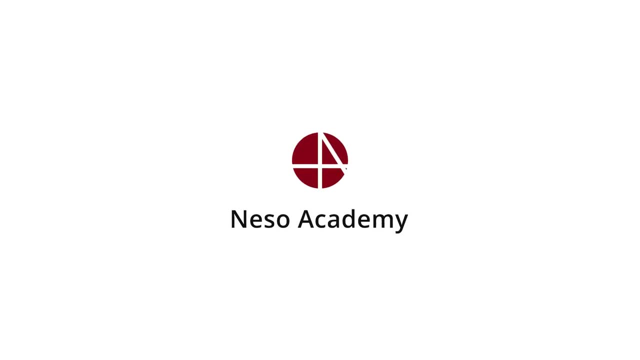 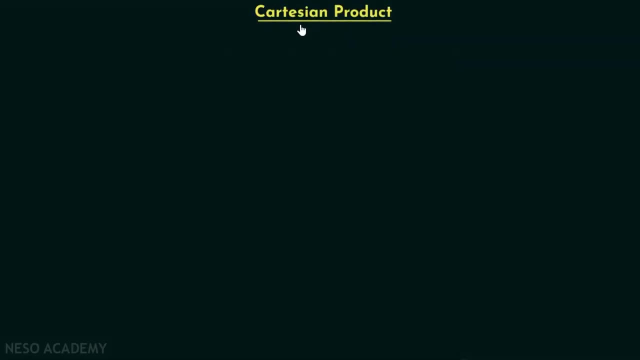 In this presentation we will try to understand this very important topic that is Cartesian product. So let's get started. Sometimes we want a collection of ordered pairs, right? Sometimes we are interested in finding a collection of ordered pairs. Let's say we are interested in. 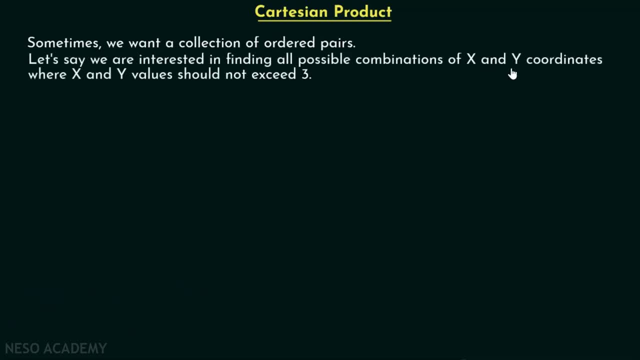 finding all possible combinations of x and y coordinates where x and y values should not exceed 3,. okay, We are interested in finding all possible combinations of x and y. That means we are interested in pairs. We want all possible combination of the pairs x and y where the values 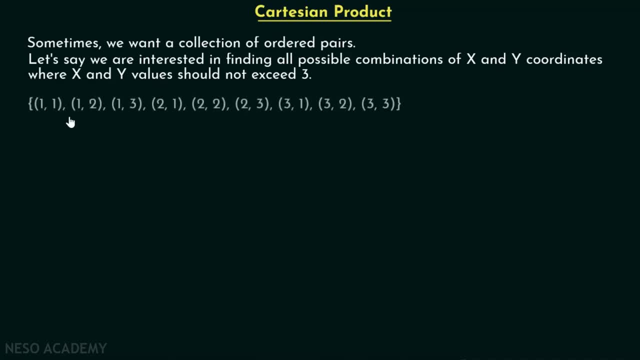 of x and y should not exceed 3.. And this is how the collection looks like. Here we have all these pairs where the first value of this pair represents the value of x and second value of the pair represents value of y. Here you can see, this pair consists of: 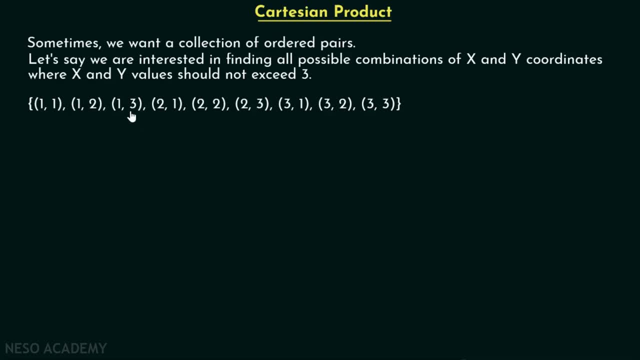 two pairs of x and y. So we want to find all possible combinations of x and y. Let's say we have two values, that is, 1, 1.. Then we have 1, 2, 1, 3, 2, 1, 2, 2, 2, 3, 3, 1, 3, 2, 3, 3.. 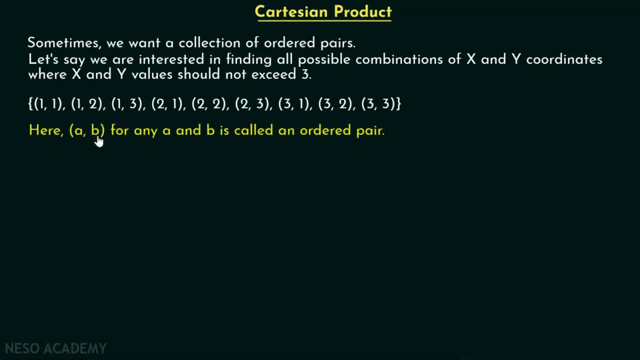 These are all the possible combinations right Here, a, b, for any a and b is called an ordered pair. okay, Now why I am calling this an ordered pair? Because let me tell you that order does matter Here. the order of a and b does matter. okay, Please note that a- b and b- a are not. 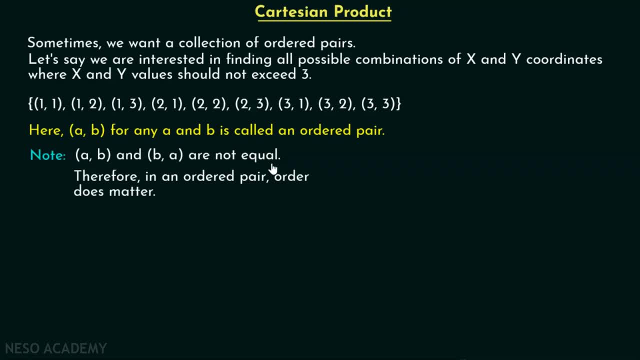 equal. Let's try to understand this with the help of an example. Why is this the case that a b is not equal to b a? Here you can see in this graph that this point is 1, 3 and this point is 3, 1.. 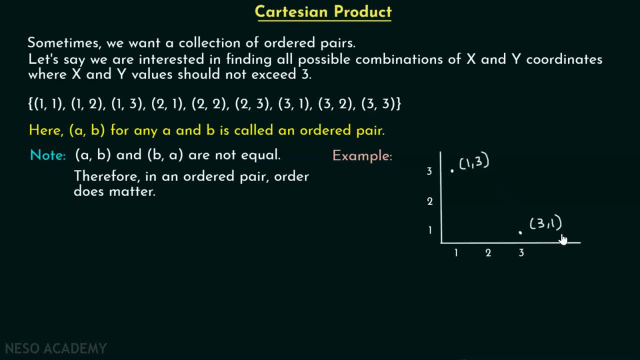 You can clearly see that 1, 3 is not equal to 3, 1.. Therefore, in an ordered pair, order does matter. okay, Now let's discuss the definition of Cartesian product. Let a and b are two sets. 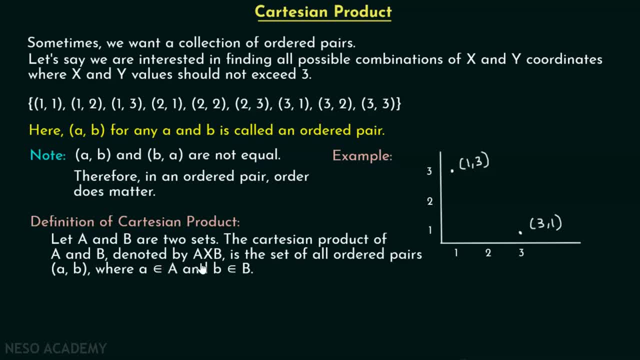 The Cartesian product of a and b denoted by a cross b is the set of all ordered pairs, a comma, b, where a belongs to capital A, that is set a, and b belongs to capital B, that is set b. In other words, we can say that a cross b is equal. 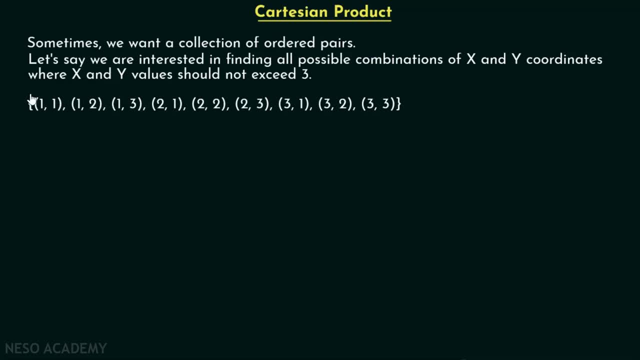 three, two, three, three. These are all the possible combinations. right Here, a comma b for any a and b is called an ordered pair. okay, Now why I am calling this an ordered pair? Because let me tell you that order does matter Here. the order of a and b does matter. okay, Please note that a comma b 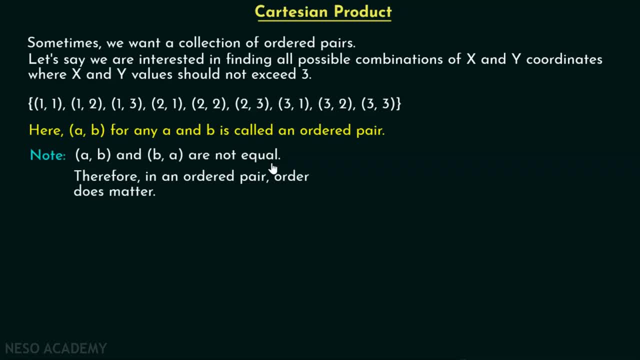 and b comma a are not ordered pairs. Please note that a comma b and b comma a are not ordered pairs, not equal. Let's try to understand this with the help of an example. Why is this the case that a- b is not equal to b a? 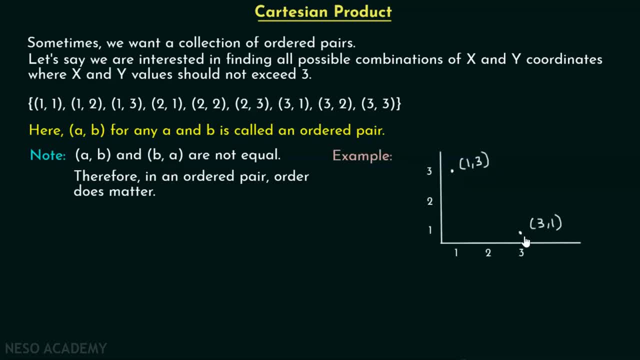 Here you can see in this graph that this point is and this point is. You can clearly see that is not equal to. Therefore, in an ordered pair, order does matter. Okay, Now let's discuss the definition of Cartesian product. Let a and b are two sets. 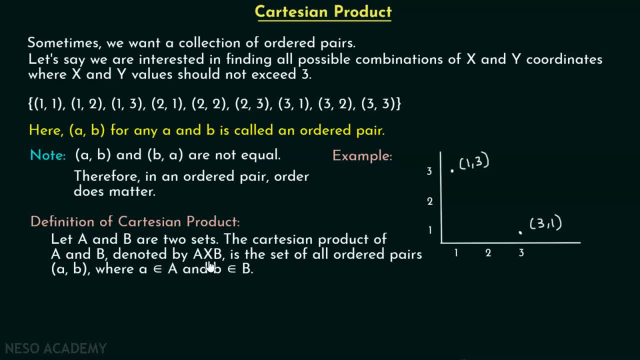 The Cartesian product of a and b denoted by a cross b is the set of all ordered pairs, a comma b, where a belongs to capital A- that is set A, and b belongs to capital B, that is set B. In other words, we can say that a cross b is equal to a set of all ordered pairs. okay. 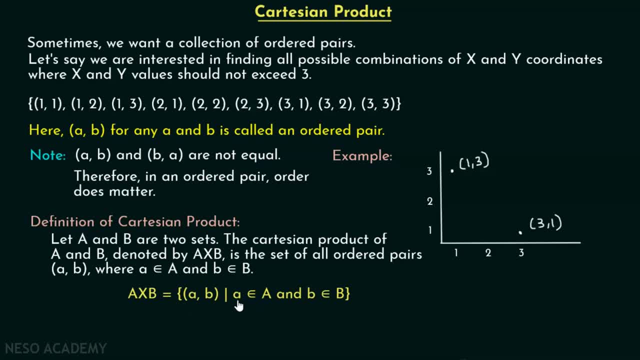 ordered pairs a, comma, b, such that small a, that is this element a, belongs to capital a, that is set A, And small b, that is this element b, belongs to capital B, that is set B. As simple as that, Okay. 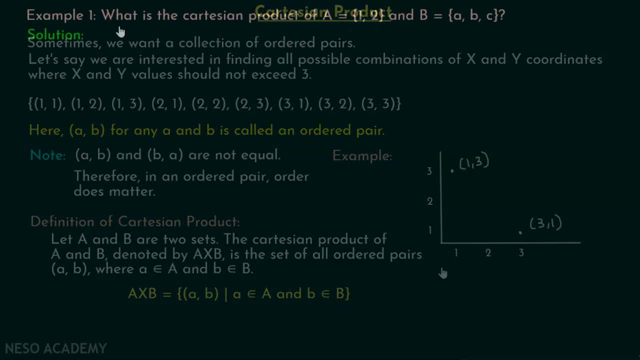 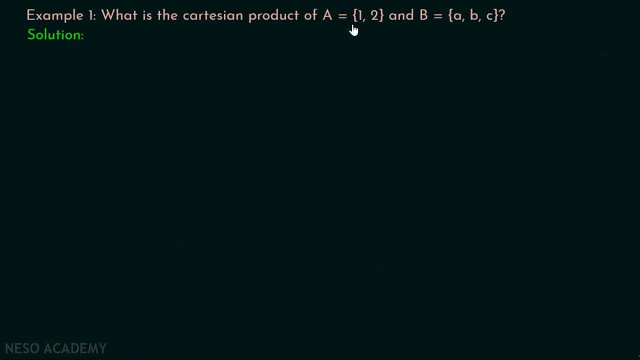 Now let's discuss one example related to Cartesian product. What is the Cartesian product of? a- that is, this set- and b- this set? Here, in this set a, we have two elements, one and two, And here in set b, we have three elements. 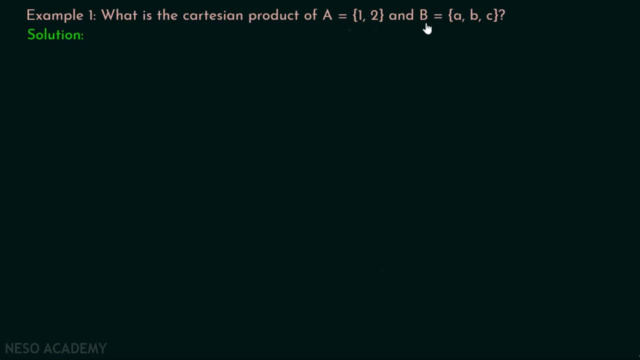 We want to find the Cartesian product of a and b. And let me tell you this is very simple. Here we want to find out a cross b. So let's find out the Cartesian product of a and b. A cross b must be equal to. we can form all the different combinations. 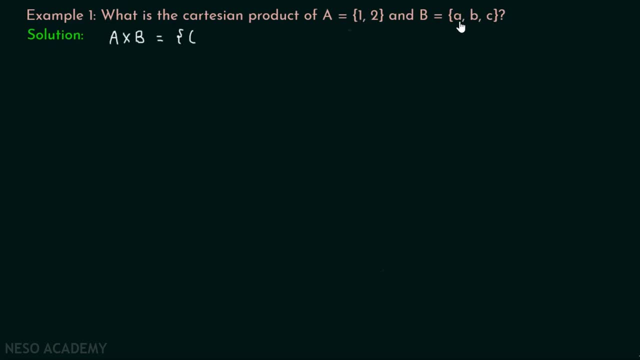 We can take the first element of a and we will take all the elements of b. Here you can see that we can take one as the first element, and second element can be a. We can take one in the first place and b in the second place. 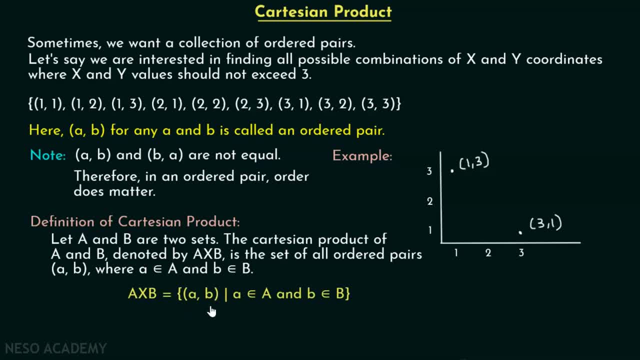 to a set of all ordered pairs. okay, Ordered pairs: a, comma, b, such that small a, that is this element a, belongs to capital A, that is set a, and small b, that is, this element b belongs to capital B, that is set b. As simple as that, okay. Now let's discuss one example related to. 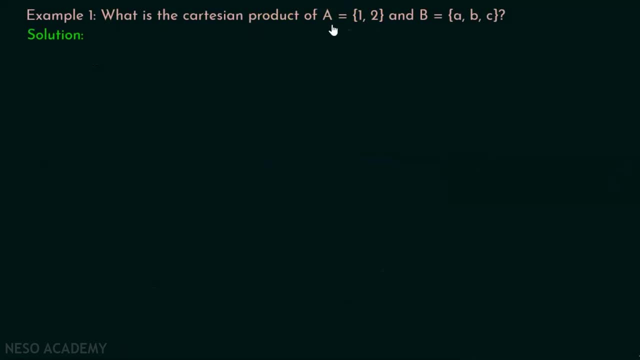 Cartesian product. What is the Cartesian product of a- that is, this set- and b- this set? Here in this set a, we have two elements, 1 and 2, and here in set b, we have three elements We want. 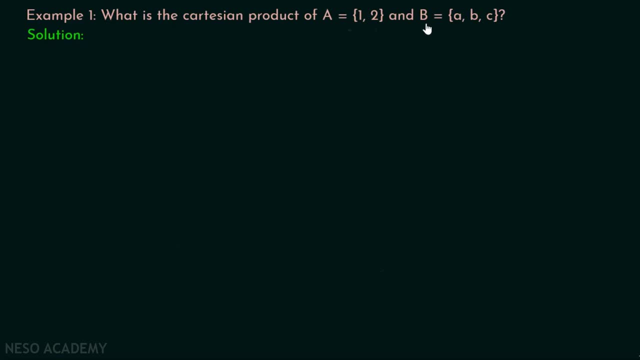 to find the Cartesian product of a and b. And let me tell you, this is very simple. Here we want to find out a cross b. right. a cross b must be equal to. we can form all the different combinations. We can take the first element of a and we will take 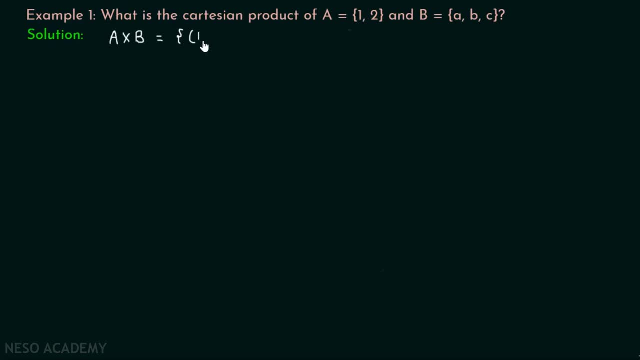 all the elements of b. Here you can see that we can take one as the first element, and second element can be a. We can take one in the first place and b in the second place, then one c. Similarly, we can have two a, we can have two b and we can have two c. So these are all the 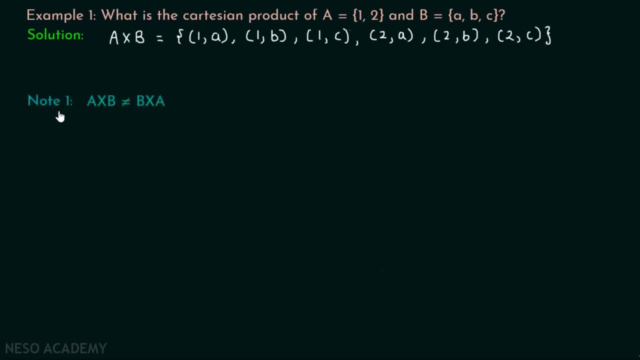 different possible combinations. right Now, here is one important thing. right Now, here is one important note: a cross b is not equal to b cross a. It should be well noted that a cross b is not equal to b cross a. Why is that so? Let's discuss this with the help of an example. Let us suppose 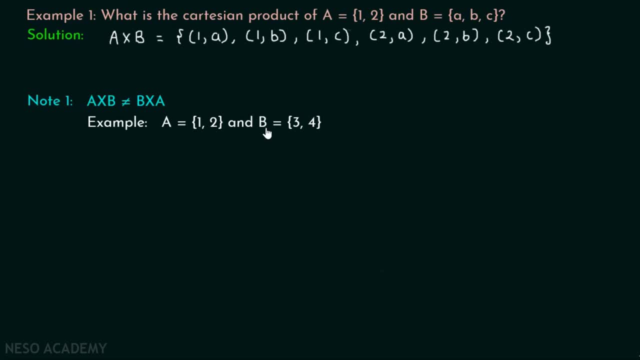 that a represents this set that is 1 comma 2, and b represents this set 3 comma 4.. What is a cross b? a cross b is equal to all possible combinations where the first element of an ordered pair must be. 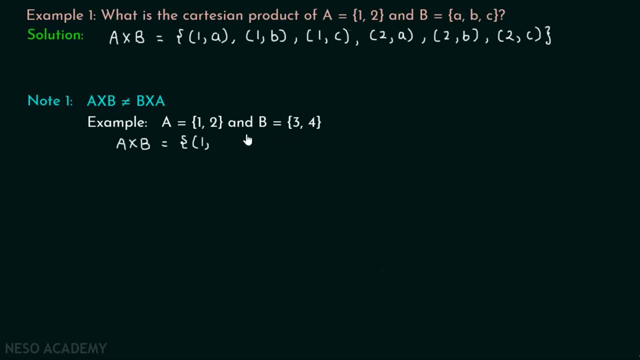 an element of a, and second element must be a cross b. So this is the first element of an ordered pair. We can have 1, 4,, then we can have 2, 3, 2, 4, right? These are all the possible combinations. 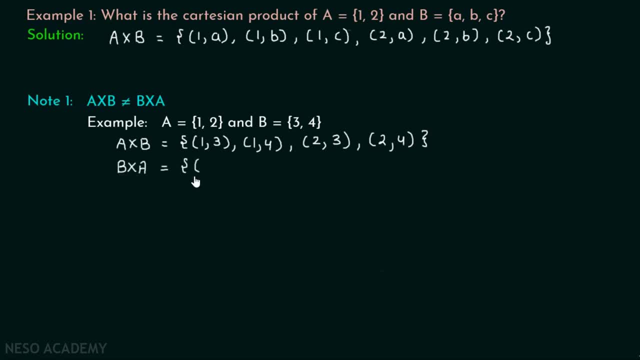 In this set we must have ordered pairs where the first element belongs to b and second element belongs to a. Let's take the first element, 3, and second element: we can take 1,, then we can take 2.. Now let's take the second element, that is, 4,. 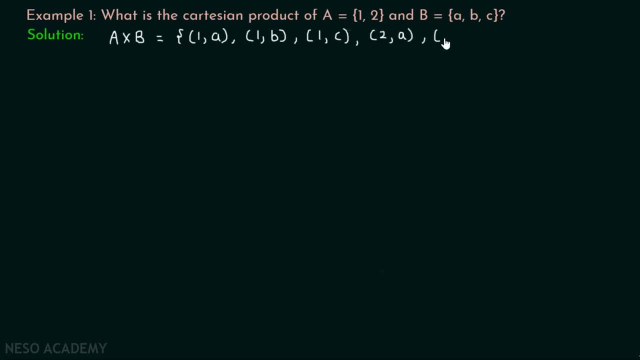 Then one c. Similarly, we can have two a, we can have two b and we can have two c. So these are all the elements. We can take all the different possible combinations right Now. here is one important note: a cross b is not equal to b cross a. 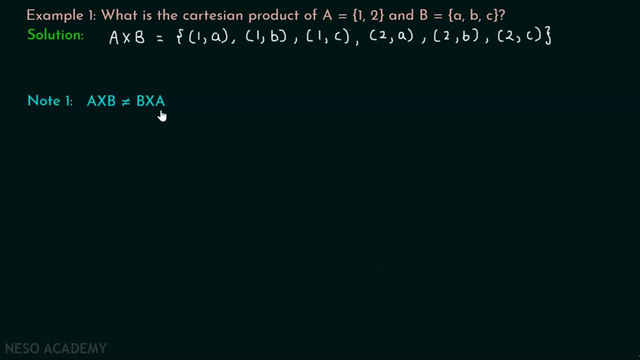 It should be well noted that a cross b is not equal to b cross a. Why is that so? Let's discuss this with the help of an example. Let us suppose that a represents this set, that is, one comma two, and b represents this: 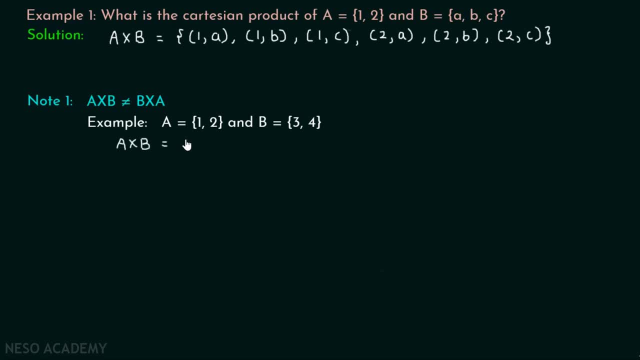 set three comma four. What is a cross b? A cross b is equal to all possible combinations where the first element of an ordered pair must be an element of a and second element must be an element of b. right, Here we can have one, four. then we can have two, three, two, four, right. 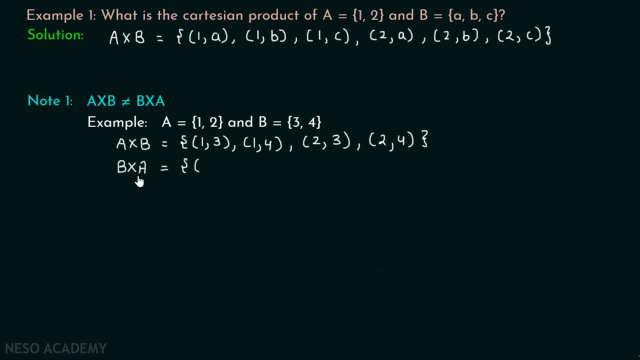 These are all the possible combinations In this set. we must have ordered pairs where the first element belongs to b and second element belongs to a. Let's take the first element, three and second element. we can take one, then we can take two. 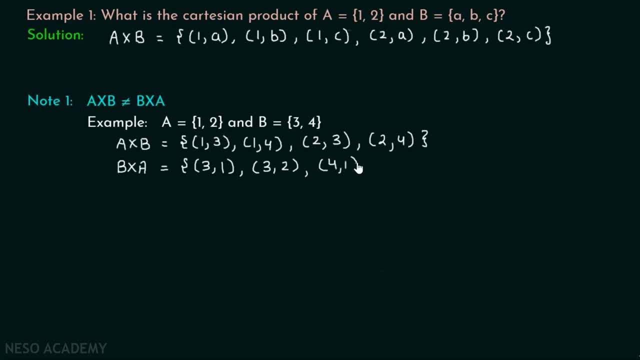 Now let's take the second element, that is, four and one. four and two. These are all the possible combinations, right? Here is one more important note: for any two non-empty sets, a and b. if there are n elements in capital A, that is set a- and m elements in b, that is set b, then the number of ordered: 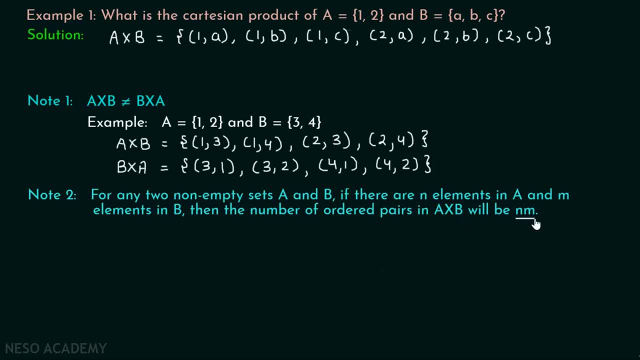 pairs in a cross b will be n m. This is very important. okay, There must be n m elements in this set. If there are n elements in capital A- that is set a and m elements in capital B that is set b, then a cross b must have n into m, that is, n m elements. 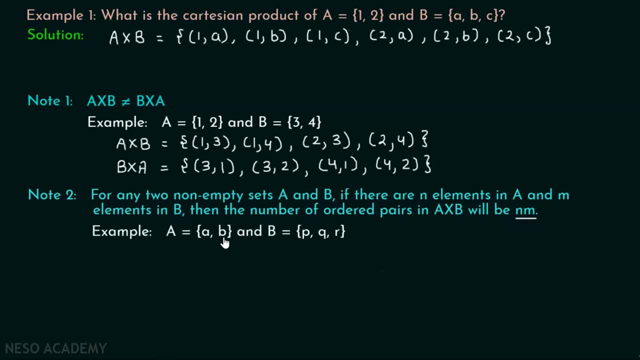 For example, we can have a set a with these elements: a comma b and set b with three elements: p, q, r. Here the number of elements in a cross b must be two into three, that is six. Why is that so? and 1,, and we can also take 2, and 4.. Now let's take 2, and 2, and 2,, and we can take 3, and 2, and 3.. four and two. 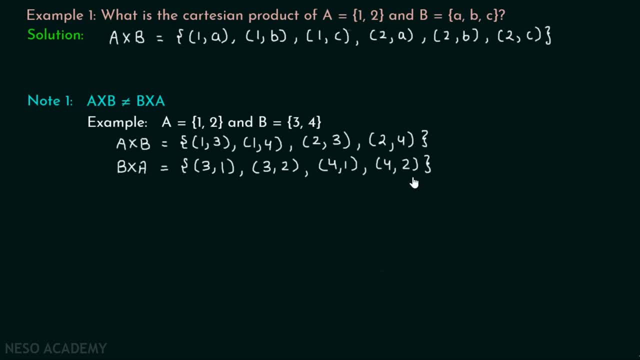 These are all the possible combinations, right? Here is one more important note For any two non-empty sets, A and B. if there are n elements in capital A, that is set A and m elements in B, that is set B. 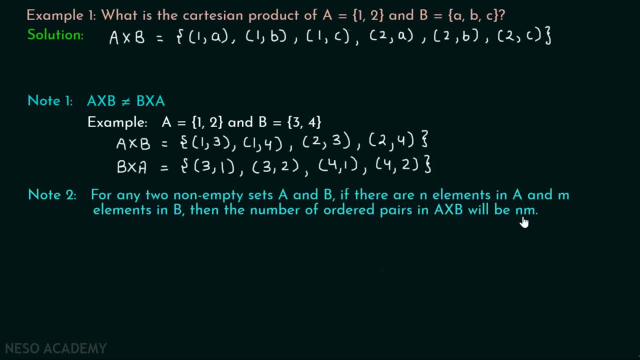 then the number of ordered pairs in A cross B will be n: m. This is very important. Okay, There must be n m elements in this A cross B set. If there are n elements in capital A, that is set A. 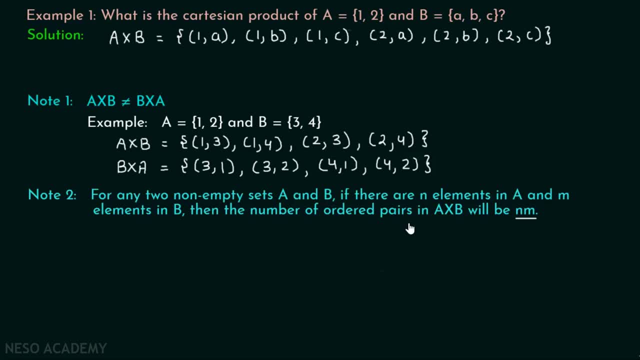 and m elements in capital B, that is set B, then A cross B must have n into m, that is n m elements. For example, we can have a set A with these elements: A, comma, B and set B with three elements. 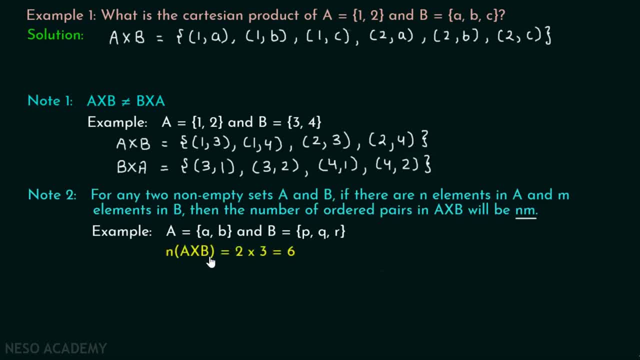 P, Q, R. Here the number of elements in A cross B must be two into three, that is six. Why is that so? We know that in an ordered pair, first element of an ordered pair must belong to the first set. 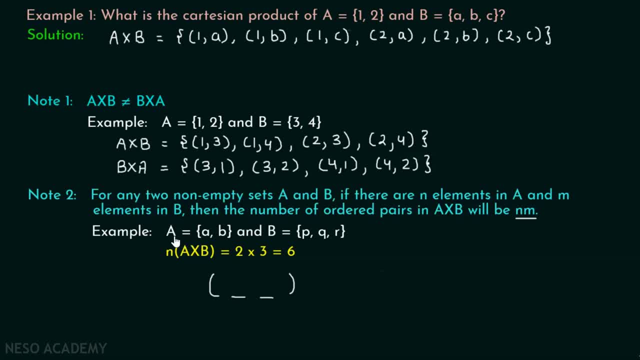 and the second element must belong to the second set. Here, in this case, we have two sets, A and B, and we are talking about A cross B. This means that the first element of an ordered pair must belong to capital A. 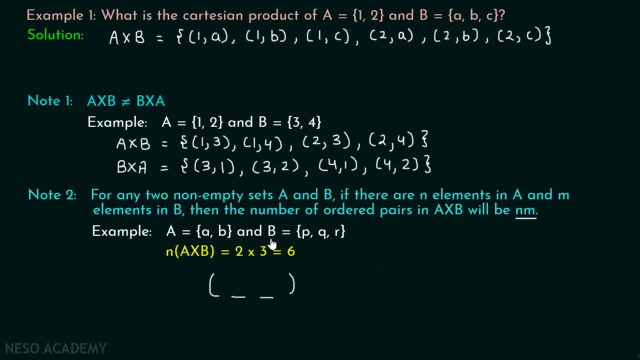 that is set A. and second element must belong to capital B, that is set B. Right, We know that there are two elements in set A, So there are two different ways in which we can fill this position, And we know that there are three elements. 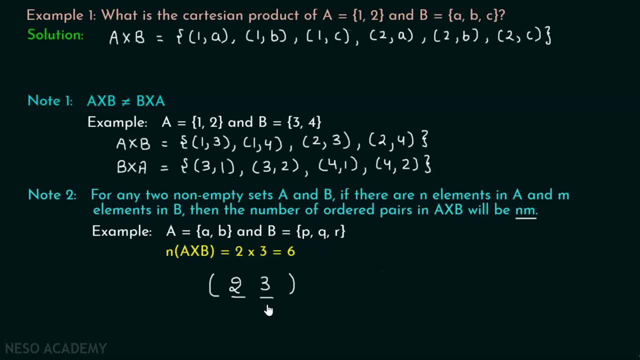 in set B. So there are total three ways in which we can fill this particular position. For every element of A we have three elements of B. So it is clear that there are total two into three, that is, six elements. 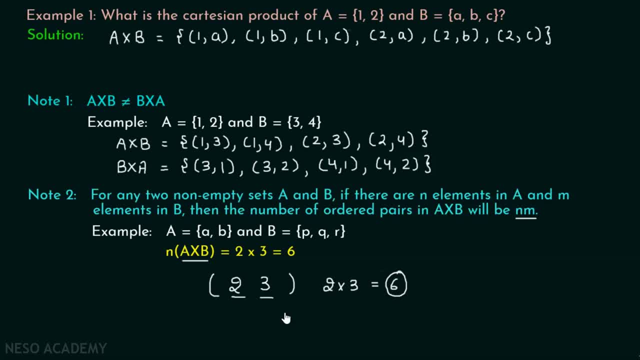 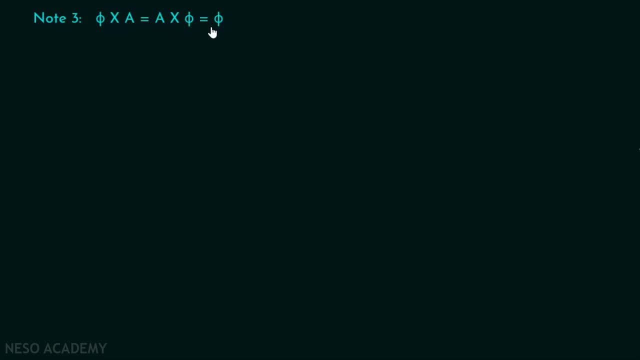 in A cross B. Right Now, let me tell you one more important point. Please note that phi, cross A is equal to A, cross phi, which is equal to phi. Why is that so? From the definition, we know that. 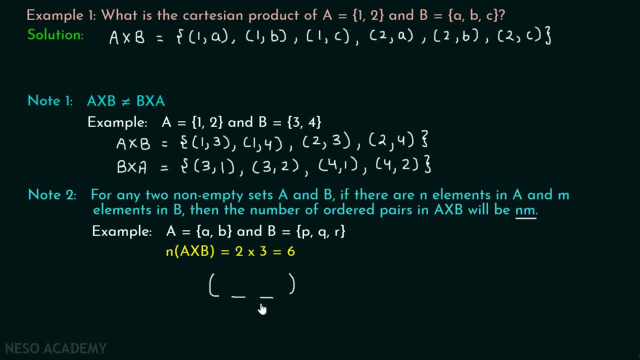 We know that in an ordered pair, set a and b must have n elements. In an ordered pair, first element of an ordered pair must belong to the first set and the second element must belong to the second set. Here, in this case, we have two sets, a and b, and we are talking about a cross b. 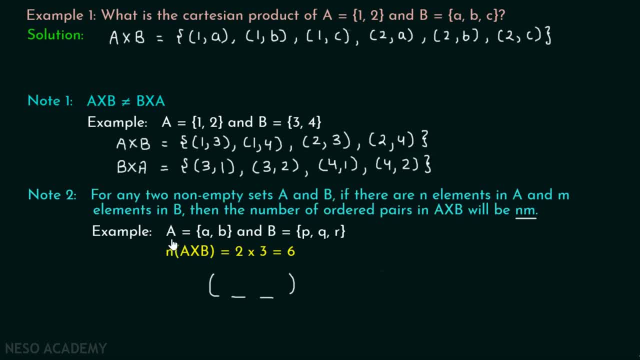 This means that the first element of an ordered pair must belong to capital A, that is set a, and second element must belong to capital B, that is set b. right, We know that there are two elements in set a, so there are two different ways in which. 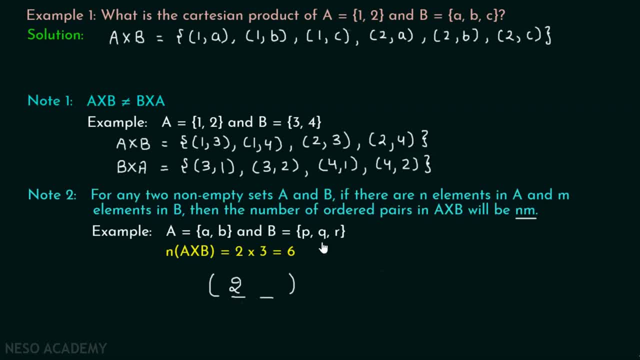 we can fill this position. We know that there are three elements in set b, so there are total three ways in which we can fill this particular position. For every element of a, we have three elements of b, so it is clear that there are total. 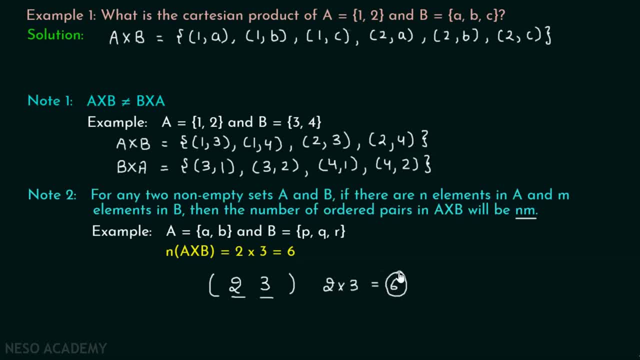 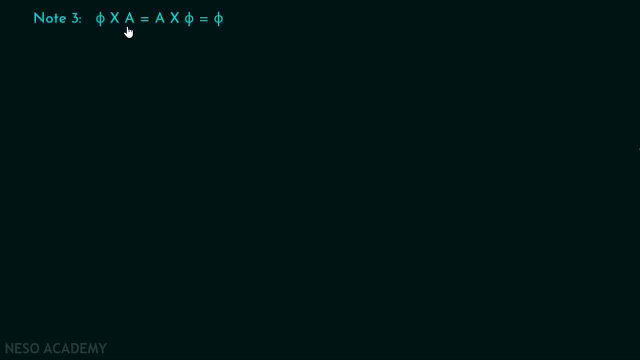 two into three, that is, six elements in a cross b. right Now, let me tell you one more important point. Please note that phi cross a is equal to a cross phi, which is equal to phi. Why is that so? From the definition, we know that phi cross a is equal to a set of all ordered pairs where 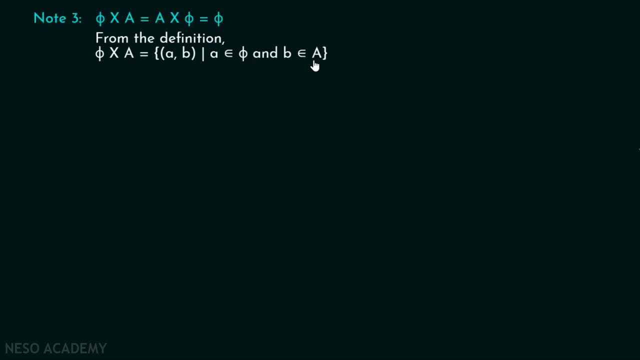 a belongs to phi and b belongs to capital A. This is from the definition of Cartesian product right Here, a must belong to phi and b must belong to capital A, because this is phi cross a. Now let me tell you that it is not possible that some element a can be a member of phi. 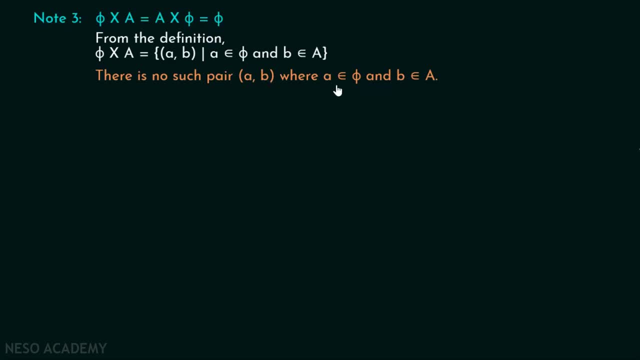 right. Therefore, there is no such pair a comma b, where a belongs to phi and b belongs to a. Thus we can say that this set is equal to phi. It is not possible, right? There is no such pair a comma b where a belongs to phi and b belongs to a. 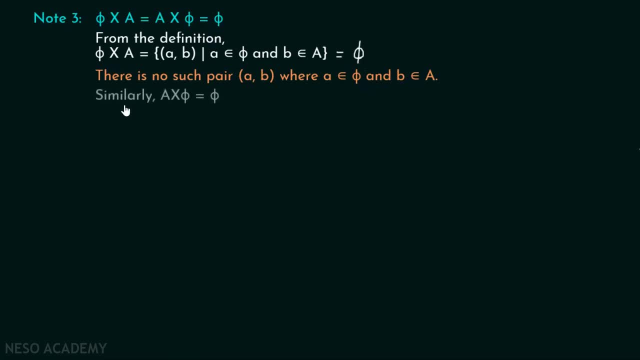 Therefore, phi cross a must be equal to phi. Similarly, we can say that a cross phi is also equal to phi, with the same reasoning Here. in this case, small b belongs to phi, and we know that there is no such small b or element that can be a member of phi.